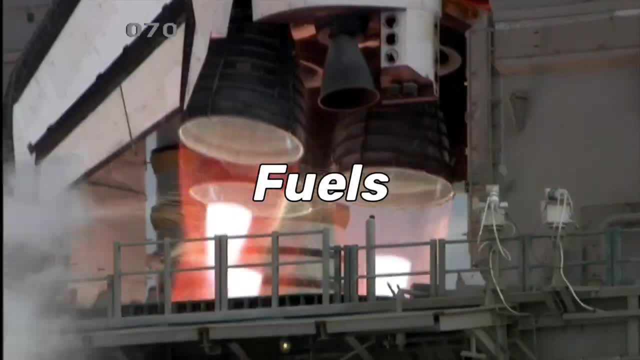 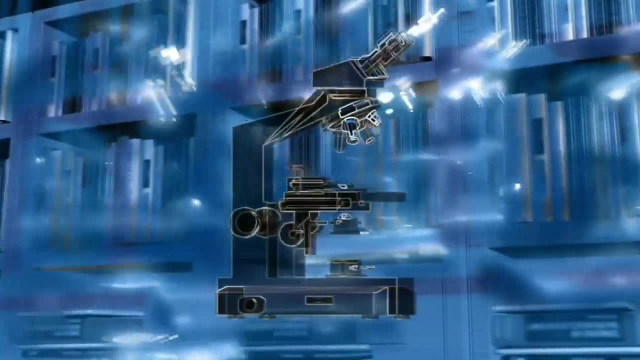 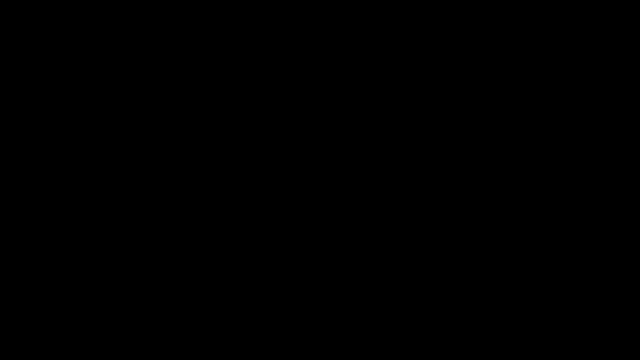 Chemical engineers work for food processing, pharmaceuticals, fuels, water and sanitation, and oil and gas industry, And now we'll head towards one of the most iconic processes in chemical engineering: separation processes. Assalamualaikum, warahmatullahi wabarakatuh, and very good morning to everyone. 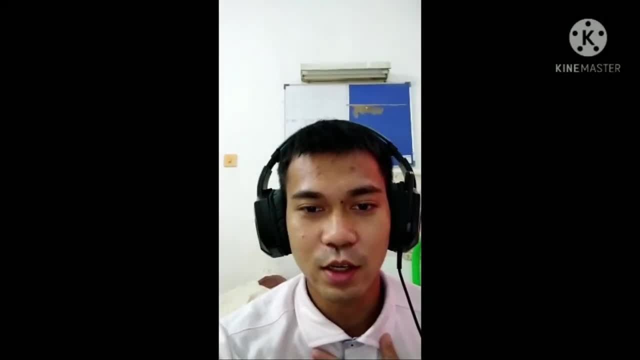 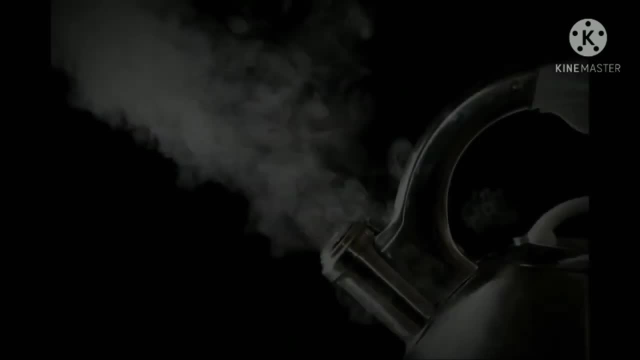 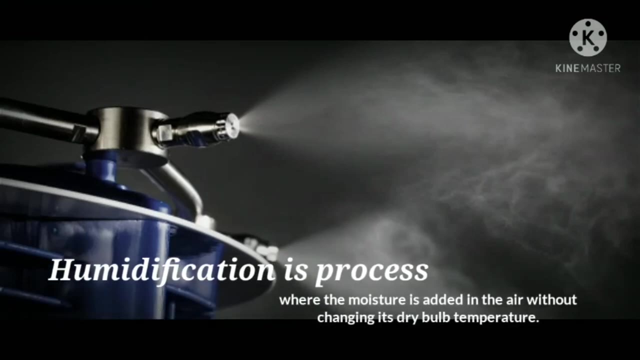 My name is Muhammad Shafiq Arifin. I'm from 4SKTK. I'm going to talk about humidification and dehumidification right now. Stay tuned, everyone. Humidification. So what is humidification? Humidification is a process where the moisture is added into the air without changing its dry bulb temperature. 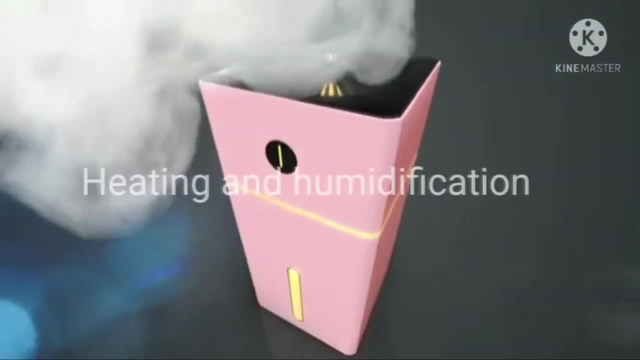 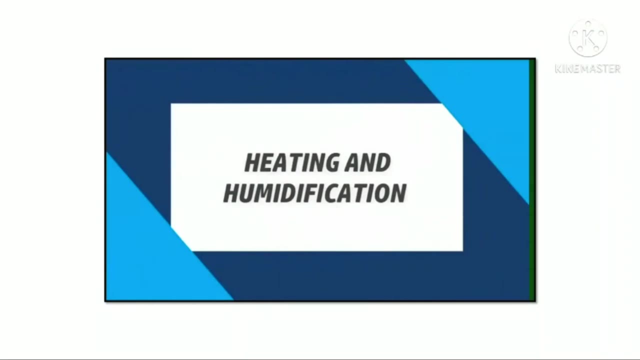 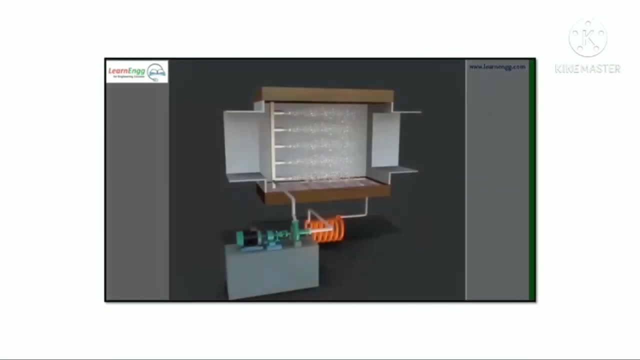 There is two types of humidification processes. The first one is heating and dehumidification, And the second one is cooling and humidification. Alright, let's take a look at the heating and humidification system. This system is oftenly used during the winter because the air is so dry and so cold. 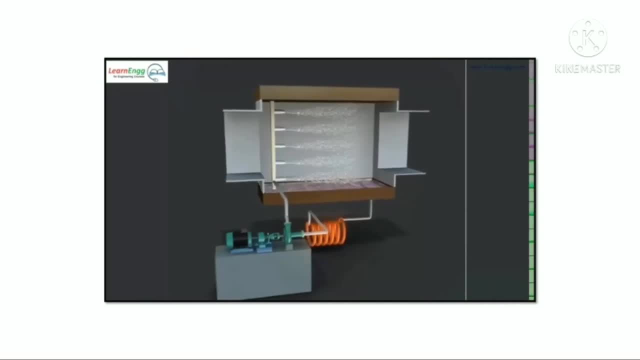 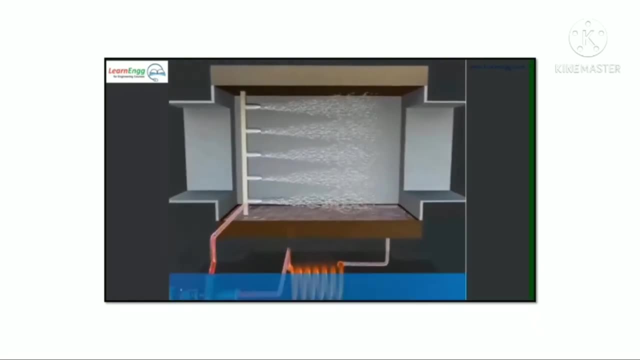 To overcome this problem, air conditioning system is used in house and cars. Firstly, the water is sprayed into the system to increase the humidity of the air. This process is controlled by using atomizer And the dry bulb temperature will not increase. Then the air is heated by using heating coil to increase the temperature of the air according to the desired temperature. 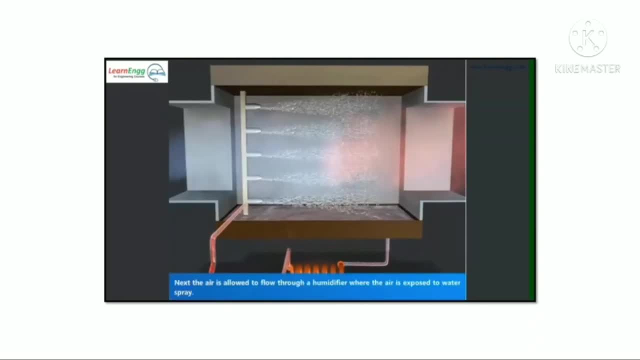 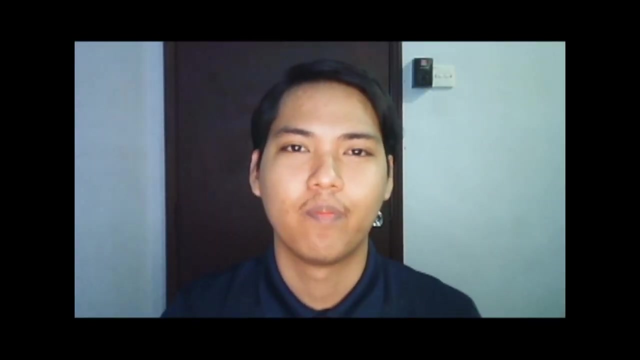 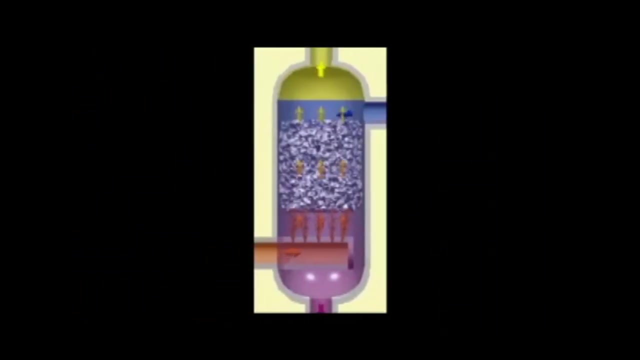 This process will increase the dry bulb temperature. Now the air is warmer and more humid. The result of this process is the house is more comfortable to live. My name is Mama Aleph, So I will continue with the absorption process. Absorption process is a chemical process in which a gas phase is connected with a liquid phase. 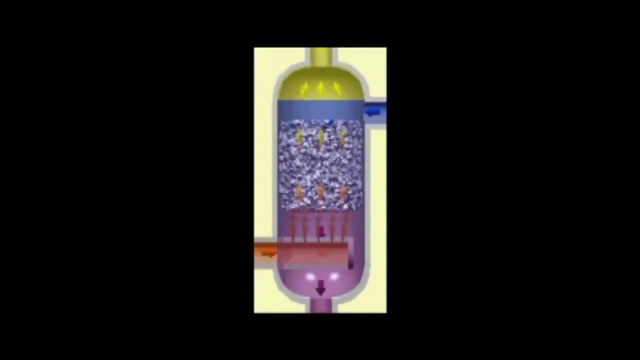 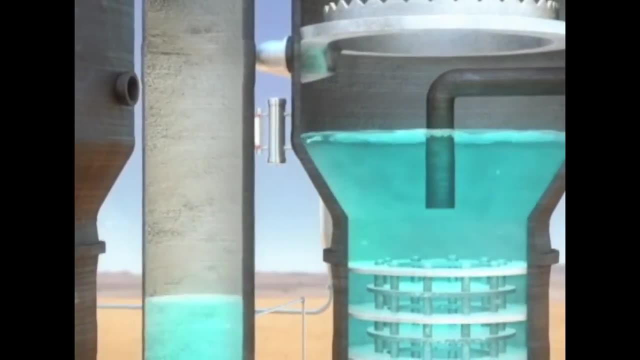 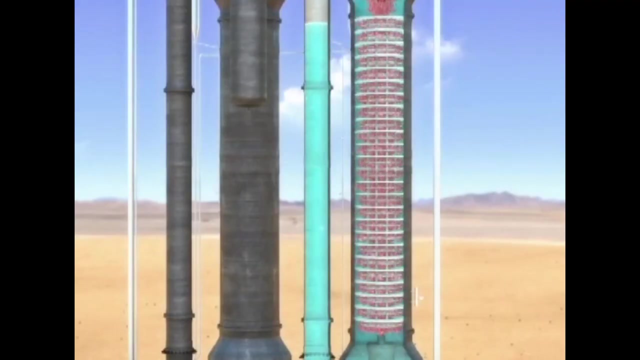 and separating one or more soluble component which is solute in the gas mixture, Then transfer a solution into a liquid phase which is solvent. The absorbable gas is then removed from the solvent and the solvent liquid stream is subsequently returned to the system. 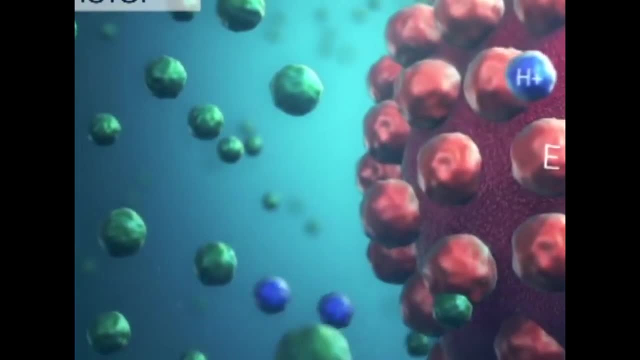 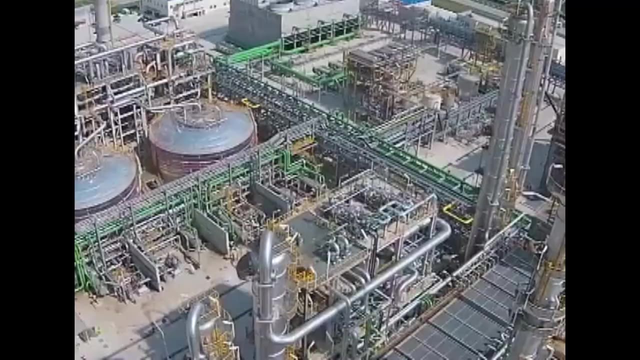 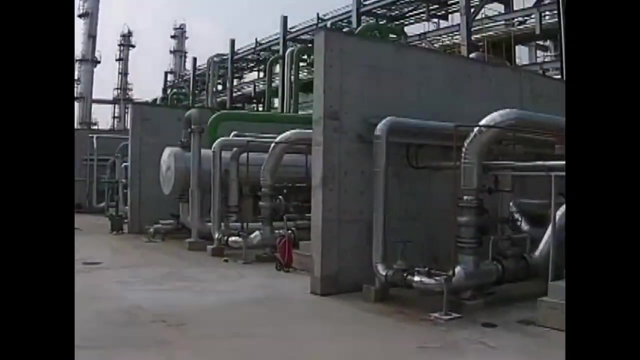 The process is called stripping. A liquid phase is immiscible in the gas phase. Its vaporization into the gas phase is small and negligible. Absorption process are widely used in the chemical and oil and gas industry. There are several examples of application for this process. 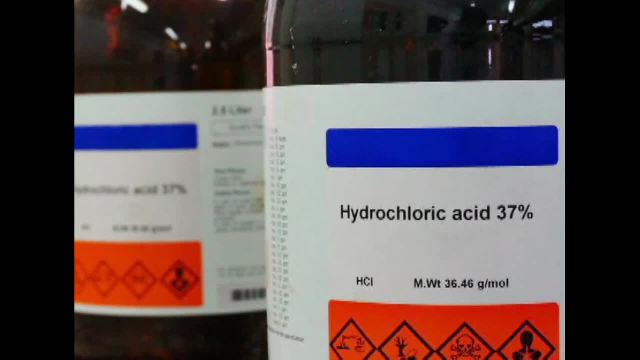 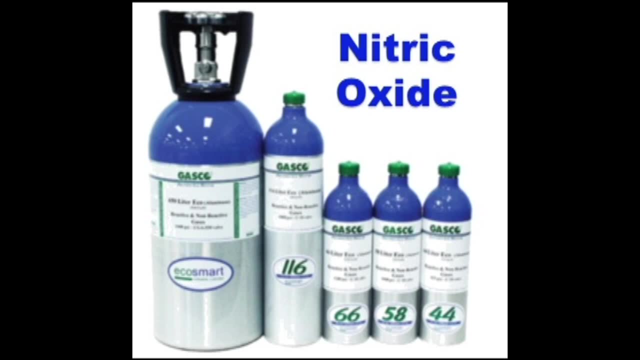 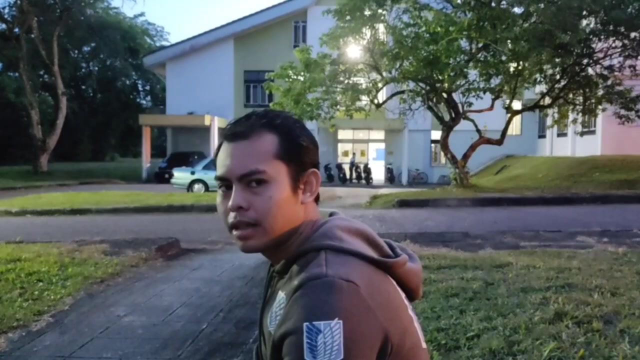 First absorbing HCl by using water in HCl production, Absorbing NO3 in HNO3 production and CO2 absorption from a greenhouse gas. Hi, I am Hafiz, and now let's talk about distillation. Distillation is a process. 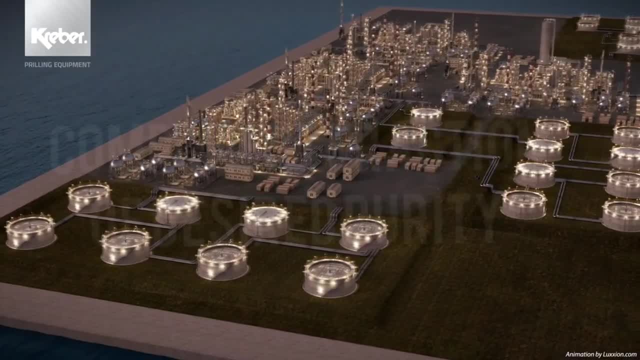 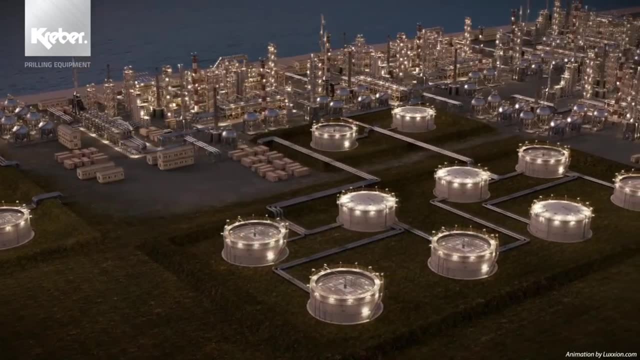 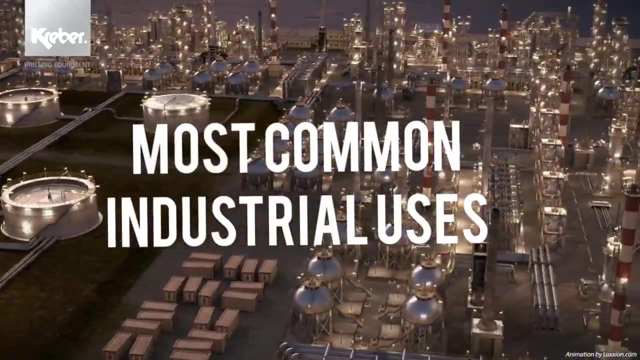 which is a liquid or vapor mixture. It is separated into its component fractions of desired purity by the application and removal of heat. The equipment used mostly are distillation columns. One of the most common industrial uses of distillation is the production of fuel from crude oils. 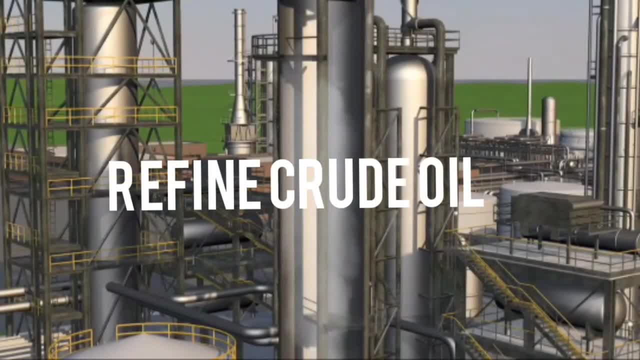 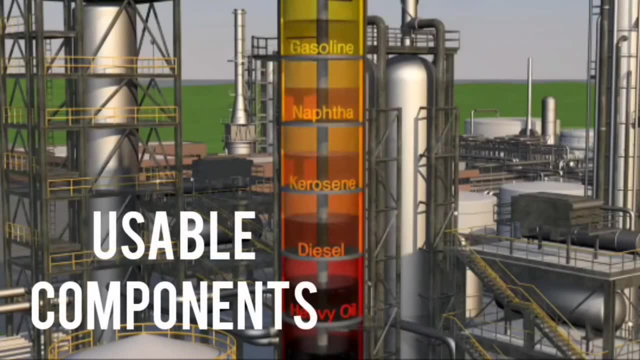 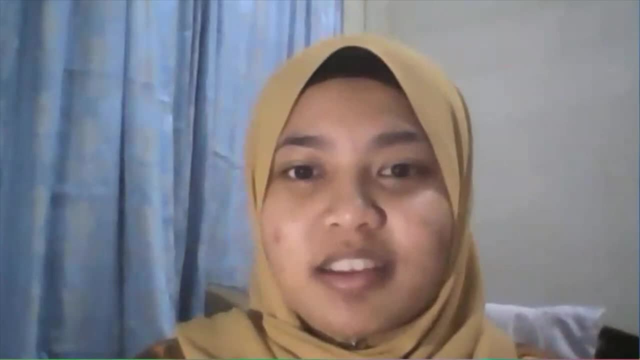 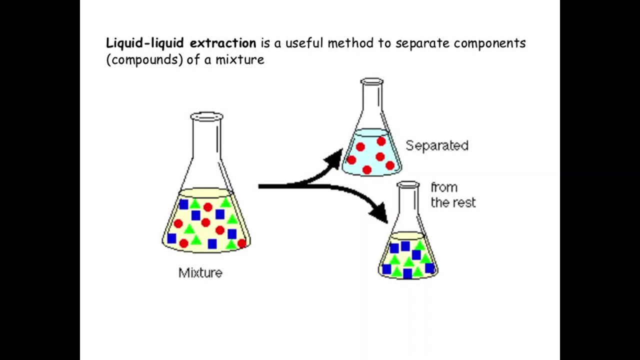 Distillation helps to refine crude oils so that fuel such as gasoline and diesel can be made from their usable components. Hi, I am Omi Zulaifa, For the next process is liquid-liquid extraction. Liquid-liquid extraction, also known as solvent extraction. 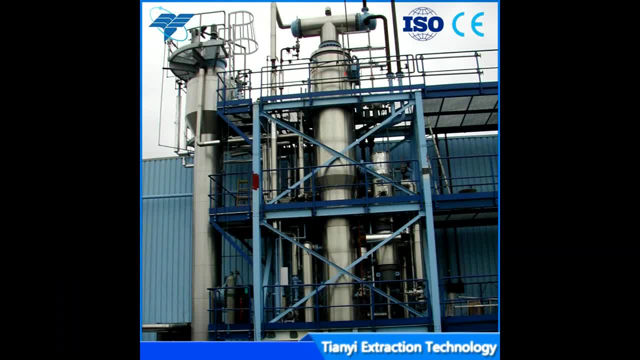 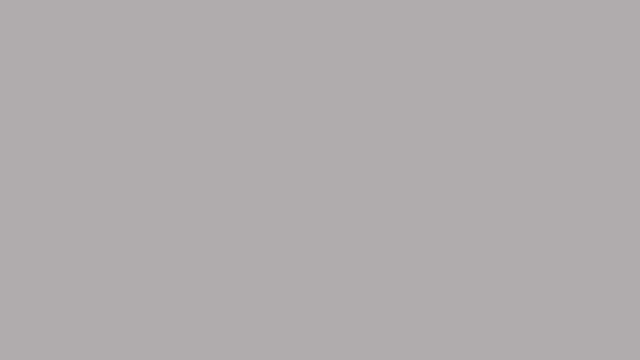 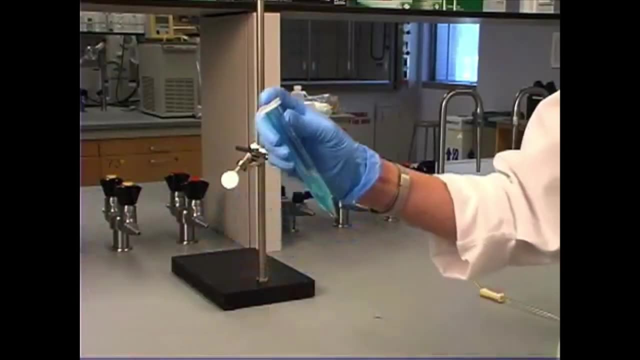 involves the separation of the solute of a liquid solution by contact with another insoluble liquid. Now let's take out this video to see how the process of liquid-liquid extraction in the laboratory works. For micro-scale extraction, firstly, mix a tube containing two immiscible layers and allow them to be separated. 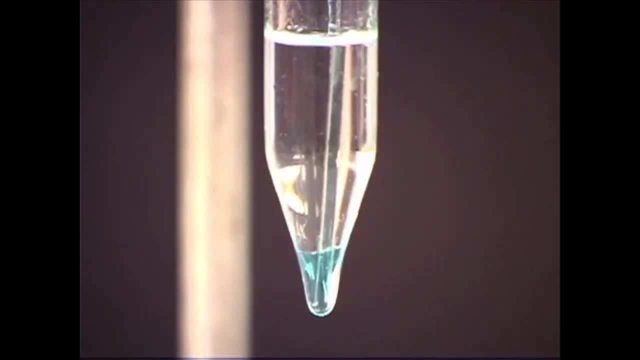 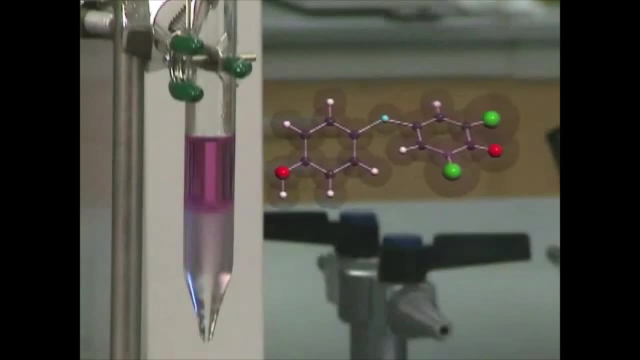 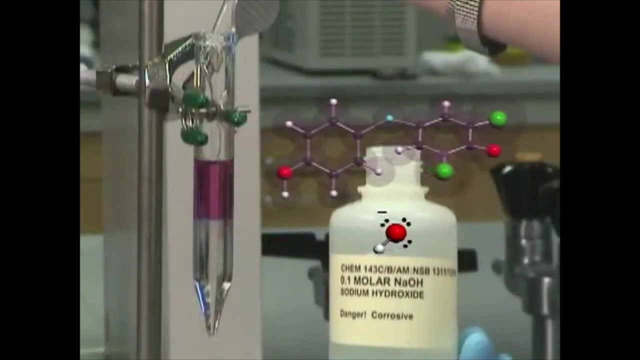 The aqueous layer can be separated from the organic layer using pipette. Always remove the bottom layer for better separation. Next, for acid-base extraction, we can move a compound between the organic and aqueous layers by changing their protonation state. The top layer contains the pink indicator. 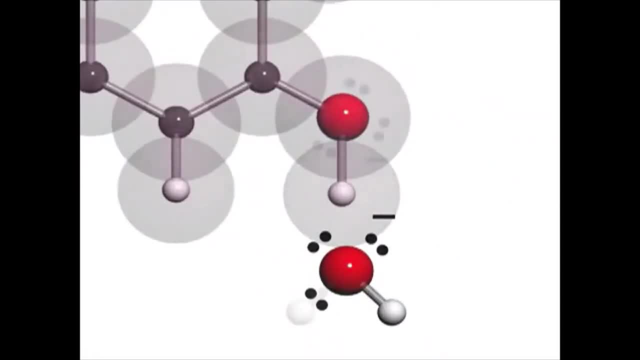 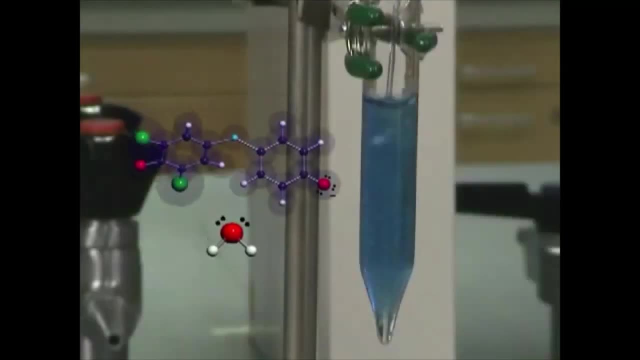 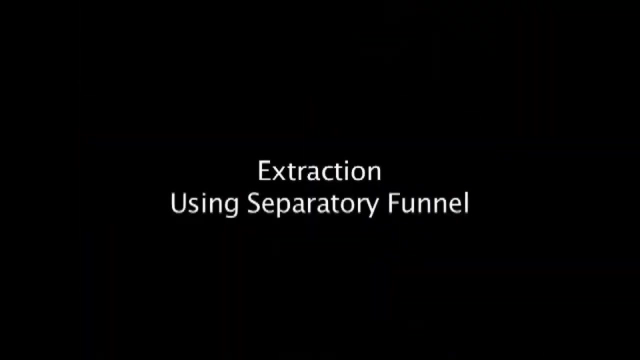 Adding base removes a proton from the indicator. The deprotonated molecule is now blue and insoluble in the bottom aqueous layer. For micro-scale extraction, a separatory funnel is used. Support the stopper with your hand. shake to mix the layer.